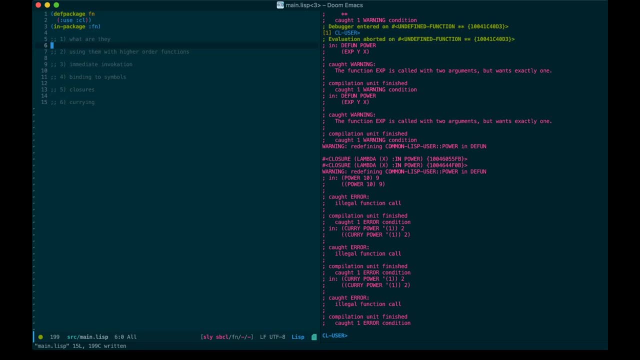 about them. They are values. In languages like this, we have functions being treated no differently from data, and especially in Common Lisp, where code is data and functions are just code. They're just, you know, objects at the end of the day. But let's have a look at the anatomy. 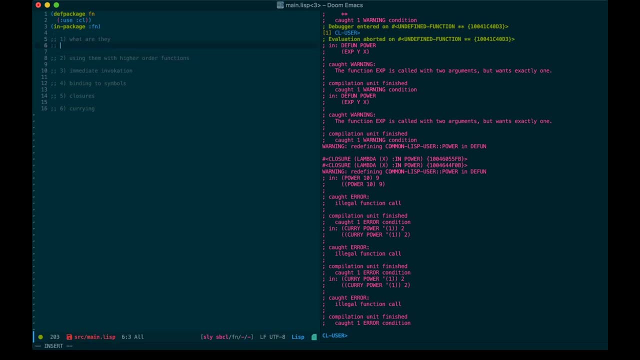 of a Lambda expression. I'm going to define a square function because they're nice and simple to remember. So we just take an x and we return the result of multiplying the x by itself, And if we print that out we get this function. 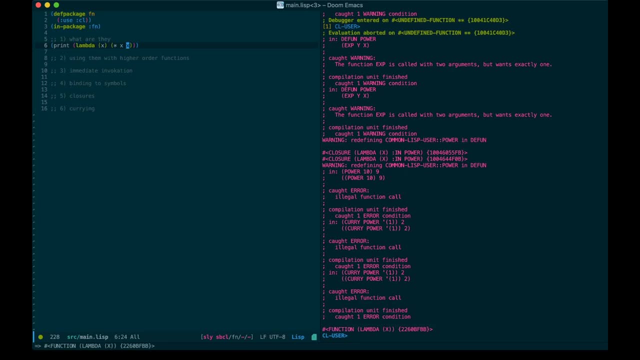 function lambda x thing here at the bottom. So this is just a value, just like anything else. They take lambda as their keyword. here We would see something like defun followed by a name. A Lambda function does not have a name, So this lambda tells us this is an. 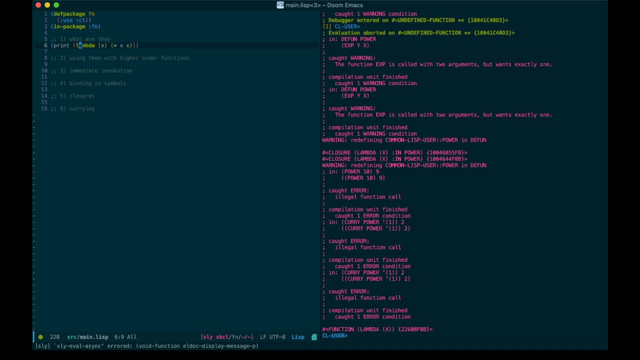 anonymous function, which is another term for Lambda functions. It's anonymous functions. You take an argument list, just like anything else, and they take a body, an expression. you know a function, body And in that respect they're exactly the same as functions. They 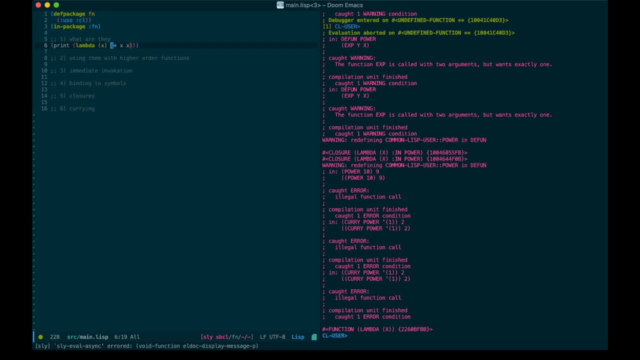 just don't have a name. Because of that, you can use them in place. We can take something like map car and we can pass in lambda And again we'll use the square And we can pass it a list of numbers and we will get our squares there at the bottom left. That one, four, nine, ten, eleven, twelve. 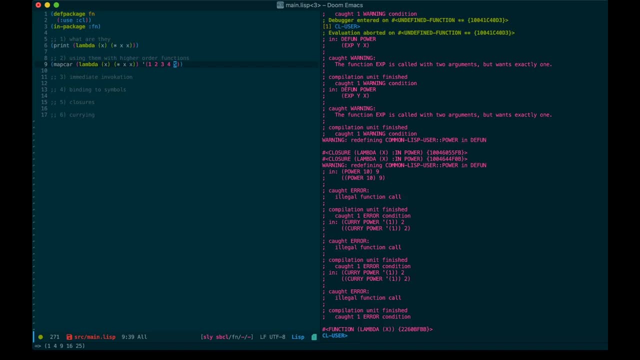 fifteen, sixteen, twenty-five. We might want to use a Lambda function here. if we're using something super simple And we don't care about reusability because it's a one-time thing and we don't want to define functions everywhere. It might be a very specialist operation and it makes no sense defining a. 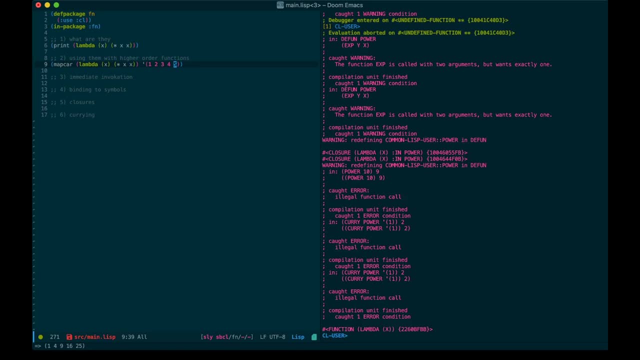 function and polluting the global namespace with that or the package namespace or whatever it is. So we might just want to use something here And we could do the same: Map car. Now we're going to say reduce, It's going to take a lambda, And because reduce takes a and a b. 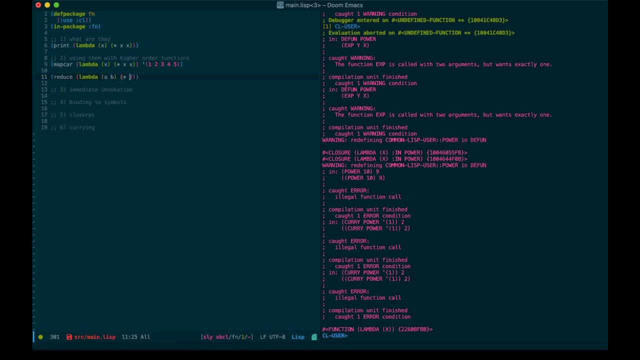 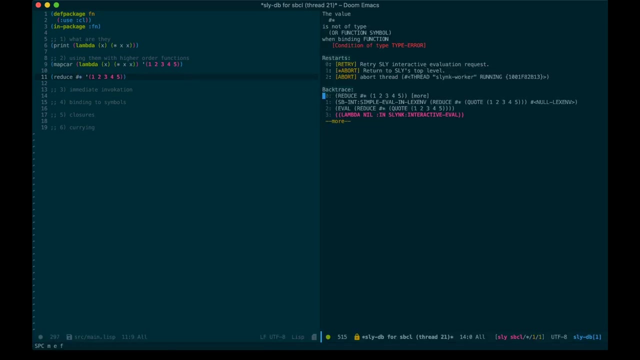 we're simply going to multiply a and b, We're going to pass in a list of one, two, three, four and five, And there we get a hundred and twenty. We had a look at this example earlier And in fact this is realistically no different from passing in. you know this, Sorry, I. 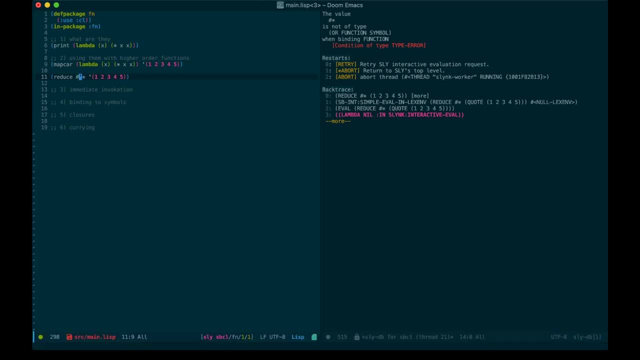 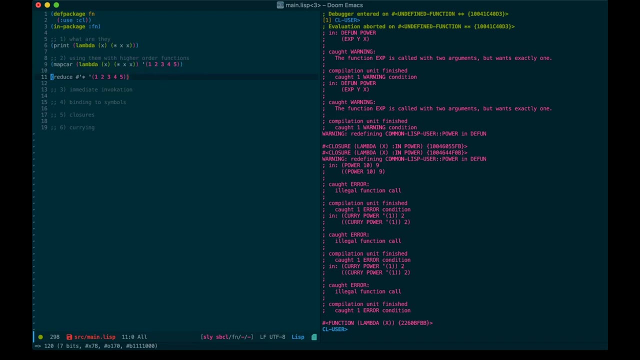 forgot a quote there. Let's abort that. There we go. It's exactly the same. But if we were going to do something a little bit more esoteric, like we multiply upon- maybe not esoteric, but we multiply upon- Let's say we add one to the result of multiplying them together, You know we get 206.. So we 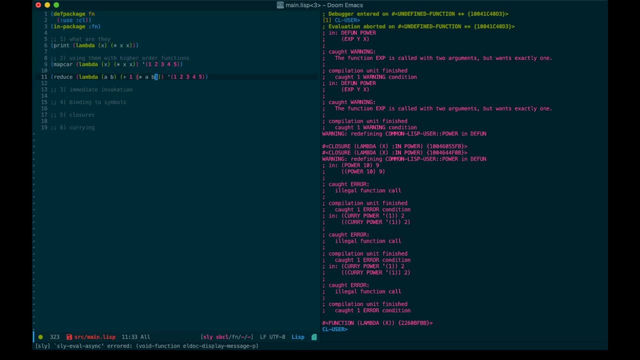 can put a specialist lambda function in here to plug into our map car and reduce functions And anything. any function that accepts a function as a parameter, a lambda can be used there. because they are. they're just functions. There's nothing inherently special about them. 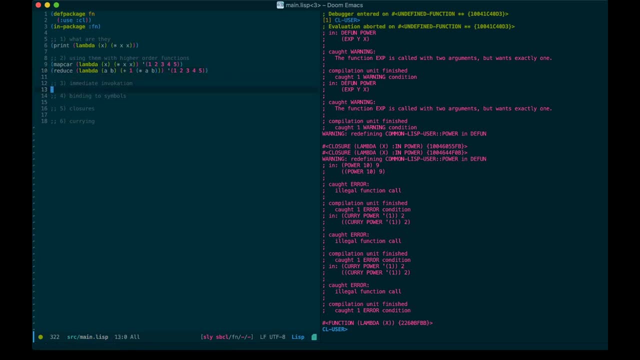 except the fact they just don't have a name, And because of that, I hope you're liking having notes here. It's helping me keep on topic a little bit. I do have a tendency to ramble and lose focus, So what we've got here is we can actually immediately invoke a function, And that might 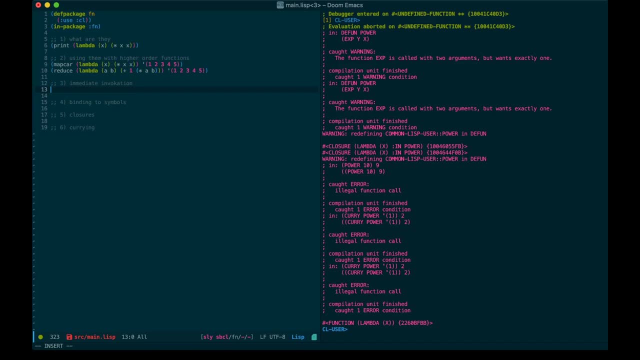 seem a little bit strange. So if I turn to my notes, because I was making notes about this, Because we know in Lisp an unquoted list. so a quoted list is one with a quote there at the beginning, but an unquoted list is a function call. in effect, We can actually 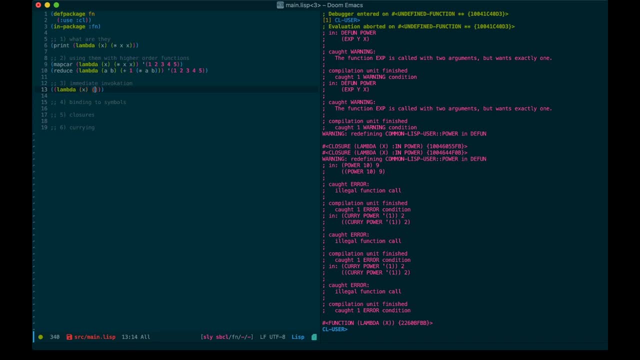 say lambda, and we'll take an x, and we will actually take a y, And we'll actually add y to itself. Now, because this is a lambda function and we're trying to invoke it, we're going to say 9 plus 9, we get 18, of course, And this is immediate invocation. So this: 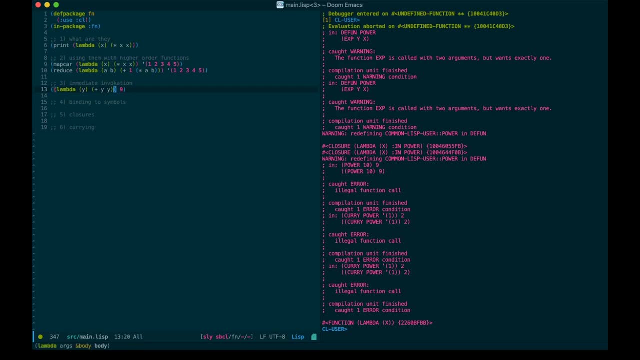 expression evaluates to a function, So that goes into the first position of our list here, So that equates to a function call And this is the second parameter, And so we can use this in place immediately. And, you know, let result be the result of this expression And we'll just print result, As you can see. 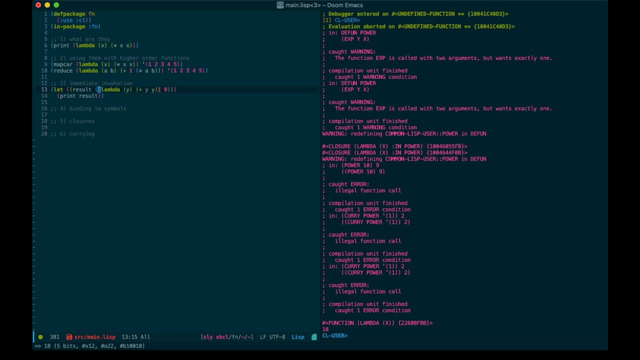 we get 18 printed out there, So that's pretty cool. You can, if you've got, you know, a complicated function that you need to calculate something, you could do it in line here just to get the results, If again, it's a one-time thing. 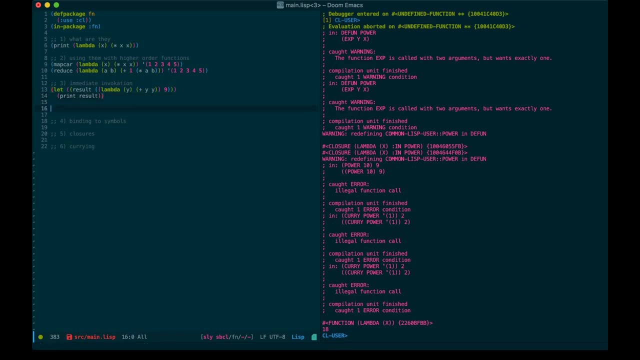 We can also chain these things. So if we again do this immediate invocation with a lambda, we're going to take a y And we're going to do the same thing, We're going to add y to itself And we return that. But instead of a second parameter, we're actually going to do a second. 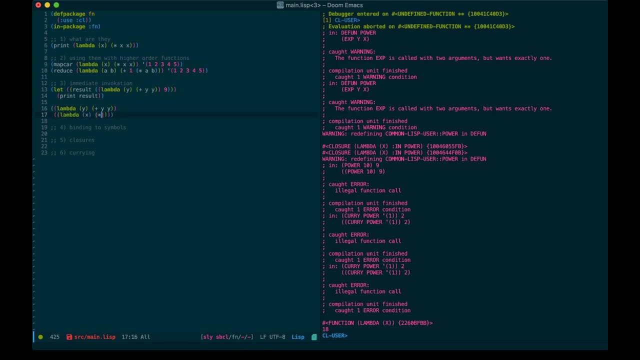 invocation. So we're going to take an x this time, We're going to square it And that is going to take a 9.. And I'm really hoping that I've got this right. There we go. Yeah, there we go. 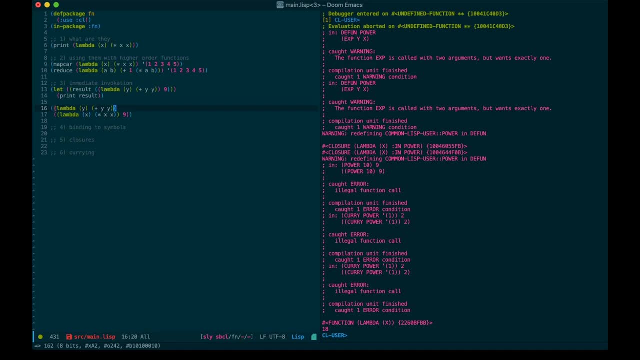 So we've got a 9. And we're going to take a 9.. And we're going to take a 9. And we're going to take a 9.. And here we are. So we actually have a 162 here. So we're taking the 9 in into the first thing here, because 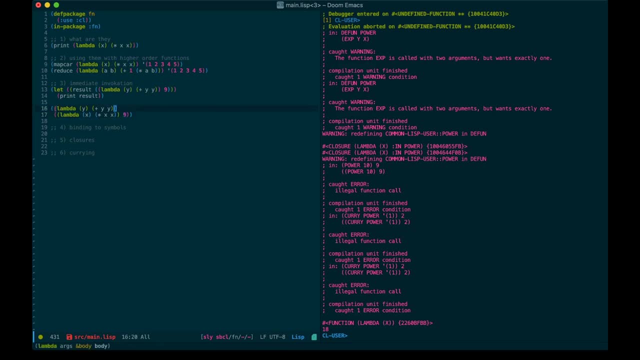 this gets evaluated as a function call because we've got these surrounding parentheses. and that goes and looks at its first argument, which is actually an immediate function call again to another lambda function here which takes an operator. So the 9 goes into here. 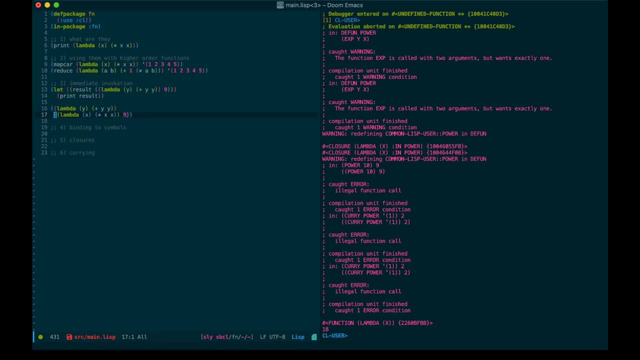 and we get 81. this evaluates and gets replaced with a value, which this function then operates on. And I'm not entirely sure, practically speaking, that you would ever use this. I certainly haven't, but because of the rules of the language, there is nothing stopping you from doing this, and in fact, 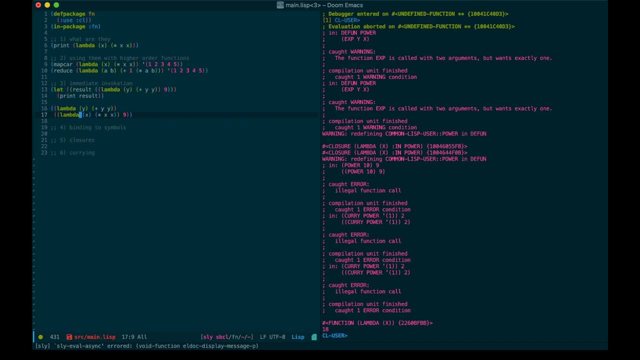 it's entirely consistent with the way the language works. We can actually do some, some interesting things here. We can actually bind these things to symbols, Def parameter. well, I'll not do a def parameter, I'll just use another, let, because lets are nicer, I think. 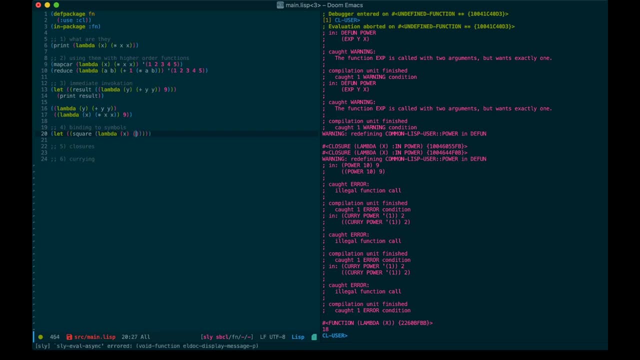 There we go. So we're actually binding this function expression, this lambda expression, to this symbol called square, and we can apply to square the list of nine and we get 81.. Remember that apply. you're applying an argument list to a function. 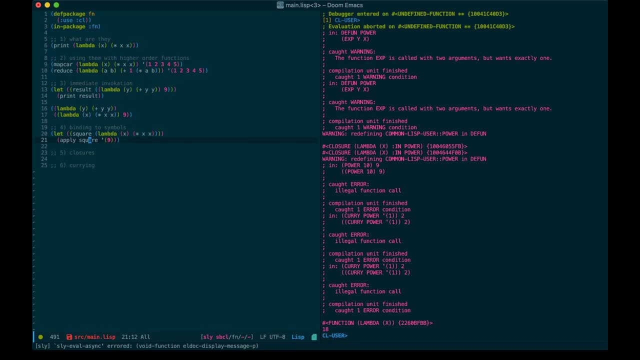 You could use func call as well if you wanted. and if you wanted to use def parameter, you could use def parameter. There's nothing about these. you're just binding a symbol to a function here. In effect, this is like a localised flet, I think. I'm not sure I'd have to investigate. 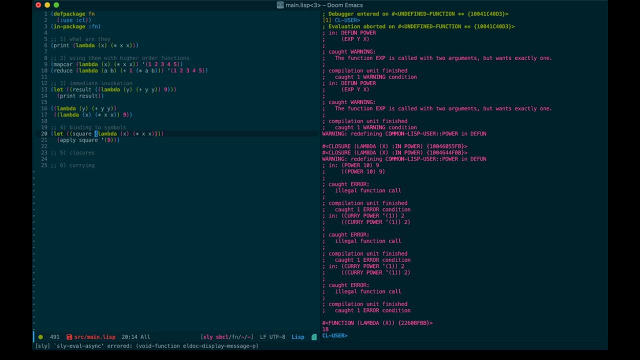 a little bit further to find out if it behaves like flet or if it behaves like labels. I'm not sure Of how the recursion would work in this context and now is not really the time to go explore and find that out. But we can also, because we can bind them to symbols we can actually have. 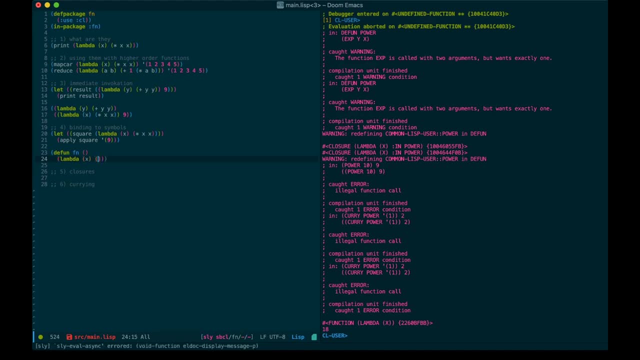 a function called fn. And again, we don't have to do anything crazy with these functions, We're just keeping it nice and simple. it's just squaring it because the behaviour of these lambda functions doesn't matter. Anything that you could do with a regular function, you can do with a lambda. 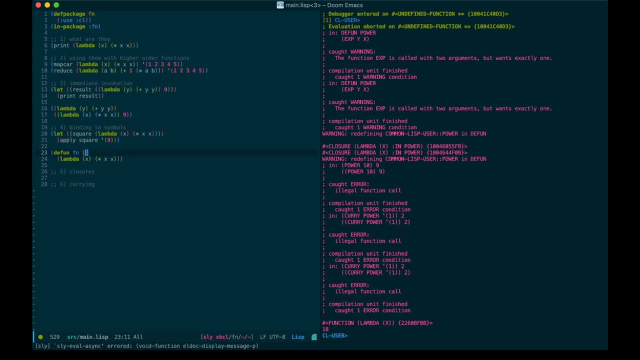 And indeed this is what actually we're doing here. We're defining a function called fn and it returns a function. So we can say: apply function. We're going to call fn and that call. what do we get? we use eight rather than nine. 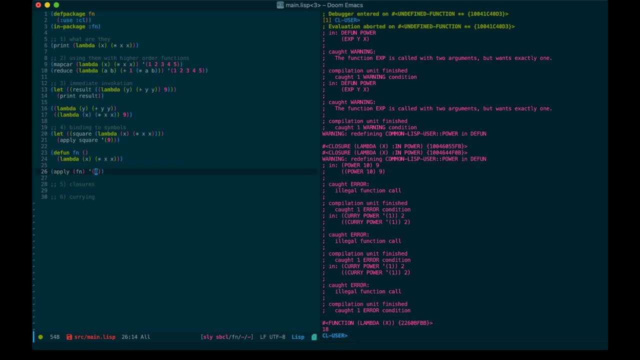 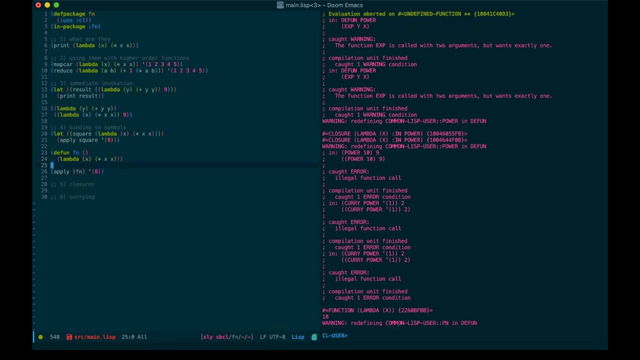 that call is going to substitute for this lambda that is doing a square here, And I will need to remember to compile that in, because that catches me out sometimes And when I do this we get 64, because when we do that we basically get this lambda function and 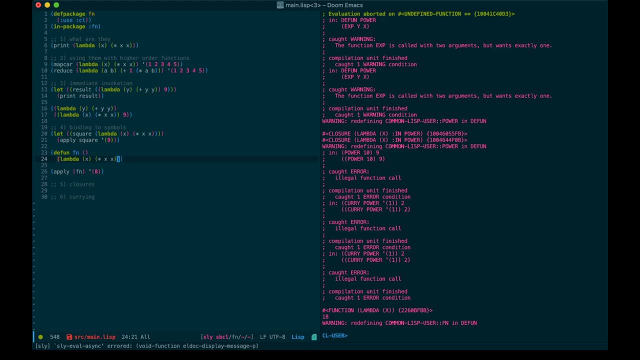 we're applying a list of eight to that lambda function, heading that back. of course we could have this. There we go. Let me remember to compile that function again. I've got an unbalanced paren somewhere. Now there we go. that fixed that Invalid number of arguments. 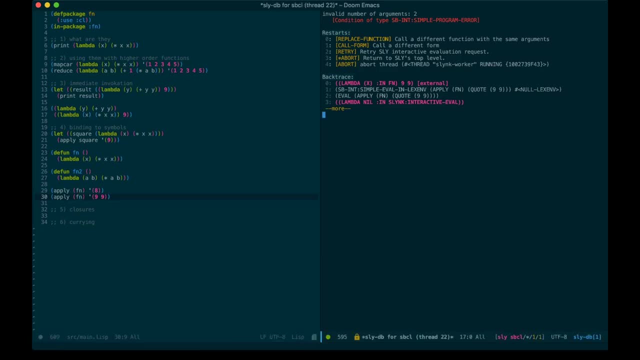 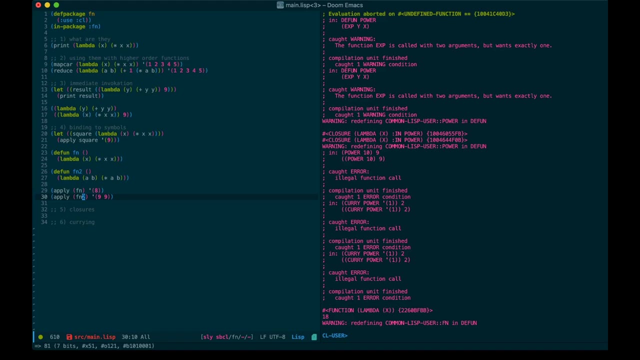 That's straight. Ah, yep, because I'm calling the wrong function, silly me. Let's put that as fn2.. There we go, so we get 81.. So again, this lambda function is accepting two parameters and we're applying a two-parameter list to the 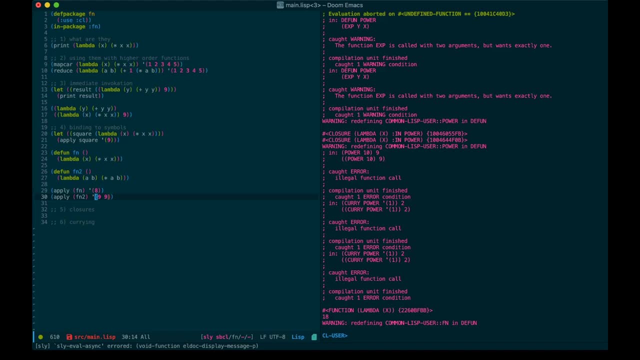 return of fn2, which returns us a lambda function. Now there's some very interesting behaviour that falls out of that, Because a function can return a function. what we can actually do is this. Let's look up a nice example here. Sorry, excuse me. 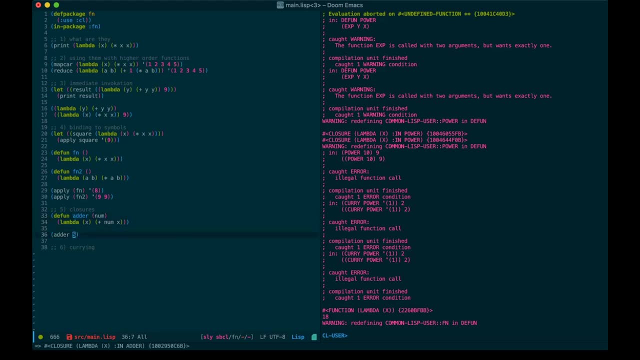 If we evaluate that, you can see at the bottom left there that we actually have this thing called a closure, which is a way of trapping state inside this function. So if we were to bind this together- let add5 be adder5, I should be able to apply add5 to the list of 5.. I might 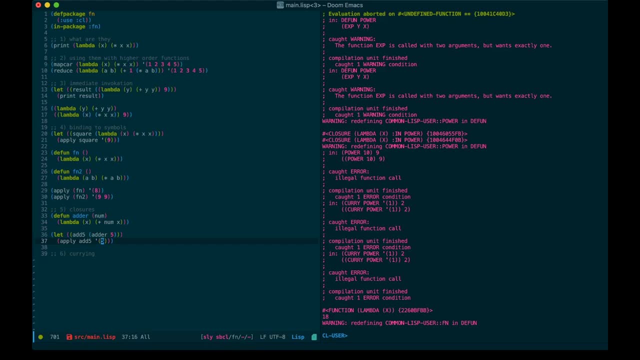 get this wrong, I might need to use the hash quote lookup. but no, there we go. We can apply add5 to the list of 5, and we are able to ensure that, no matter what we pass in here, this x, this 4, here, in the context of this, that number is always going to be bound to. 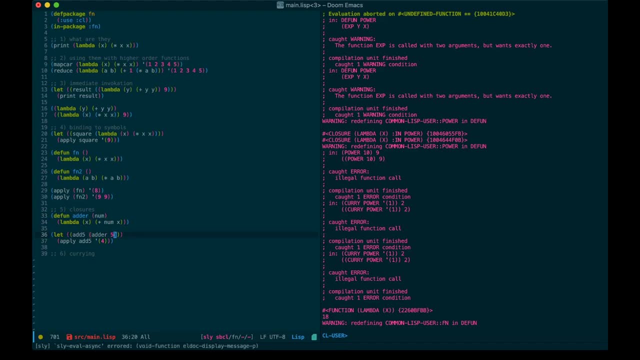 the 5 here. So this is what's called a closure, and they say that because it's closed, So it's closing over a value. It doesn't matter what this is called here. this could be like Still works The name of the symbol that's bound to. it could be anything, But we know. 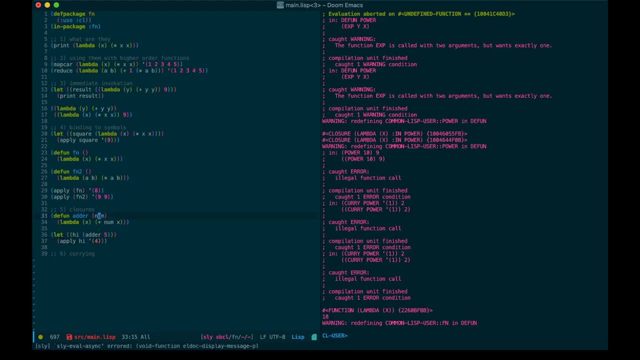 that this num, because of here, when the function, the lambda function, gets called, which is here, it's always being called when num equals 5.. We could also do this And we get 4, because in this instance we're binding a different instance, a different. 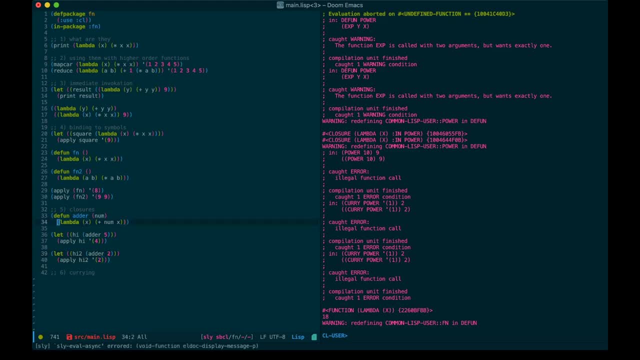 context of this lambda function to something else. And every time that we make a call to The return value value of that, we get plus two. So this is really cool and it can build on some very interesting things, which is kind of sort of what we're going to look at finally here. 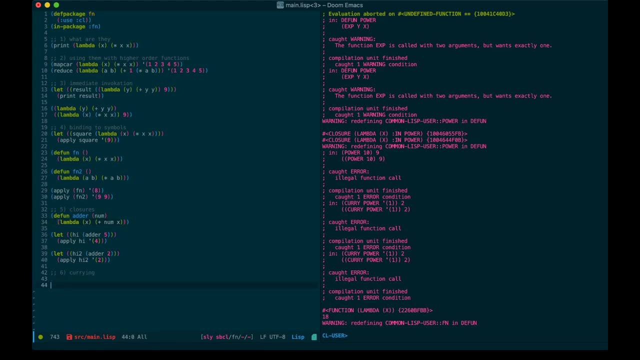 is something called a curry, And I'll just take this out. Sorry, let me pull that as far as one. So this might look a little bit more like a curry, but it's definitely not. So this might look a little bit more like a curry. So this might look a little bit more like: 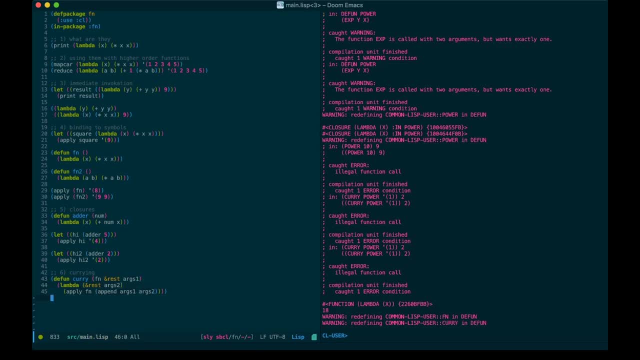 look a little crazy. We have this thing called a curry, and curry returns a function that returns something. it returns a function that is the application of another function with some extra arguments, and that sounds pretty crazy. There's a difference between currying. 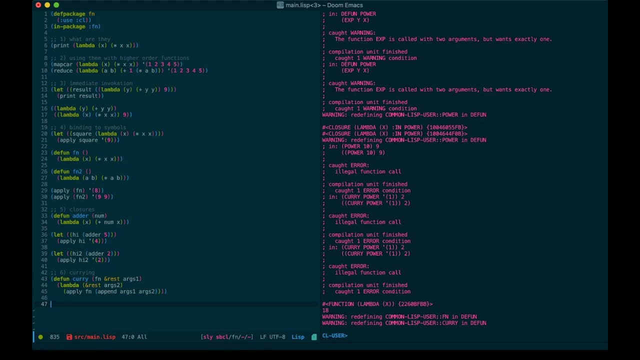 and partial function application which I can't really get into for time constraints, but trust me. Let's say we have this function called exponent, So 2 to the 3rd power is 8,, so 2 to the 4th, yep. Now what we might want to do is curry this function and that. 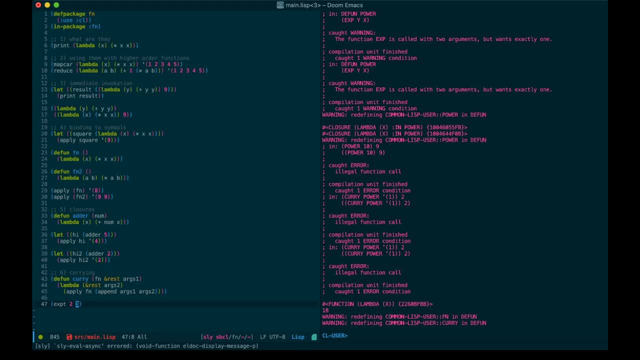 means that we can turn a function of two arguments into two functions of one argument. So we might say: There we go. it's the exponent, It's the result of curry. 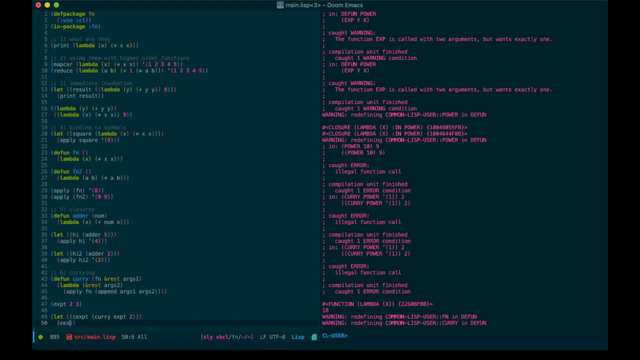 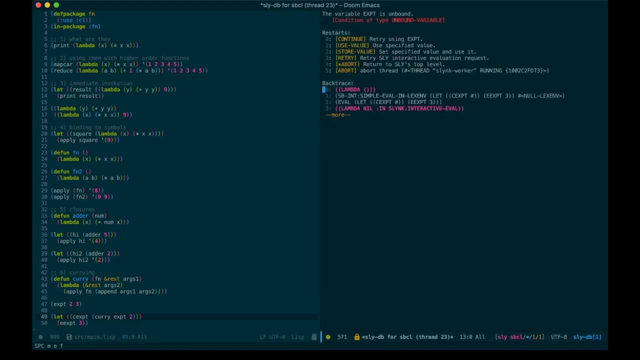 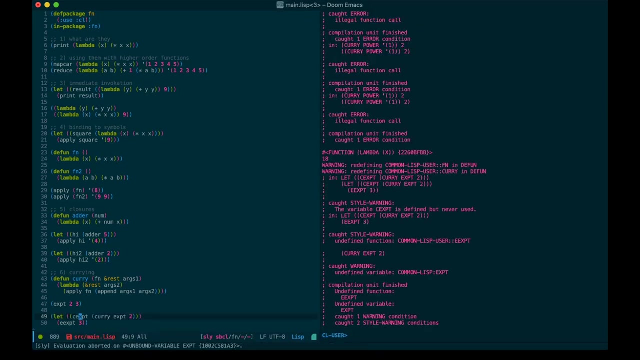 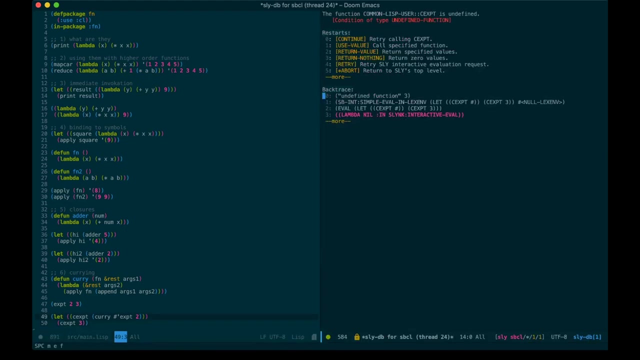 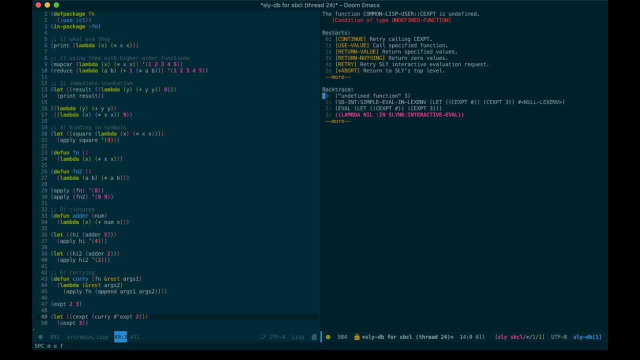 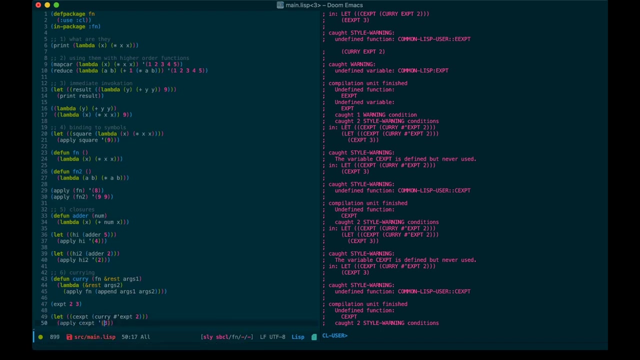 And there we go. So what we've done is we've got this function here of two arguments. 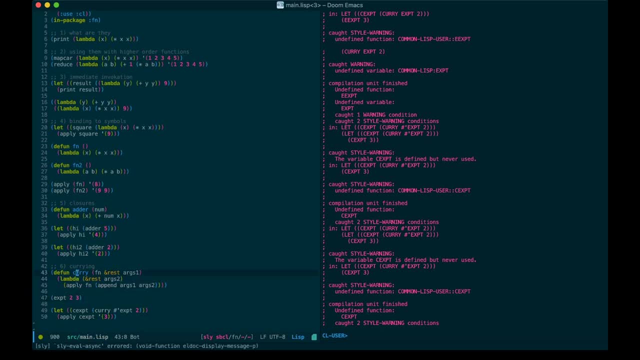 takes a base and power and with this defined curry function that we have here, which I'll break down in a minute, So we can get a new variable which is the result of currying this and it applies the arguments. Now we can do something else here. 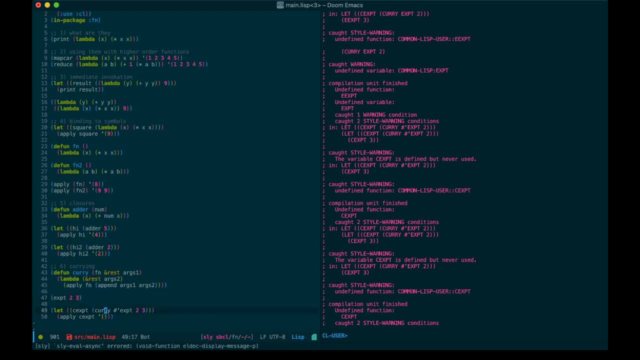 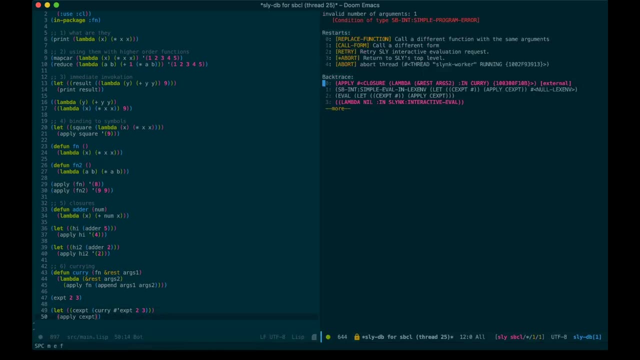 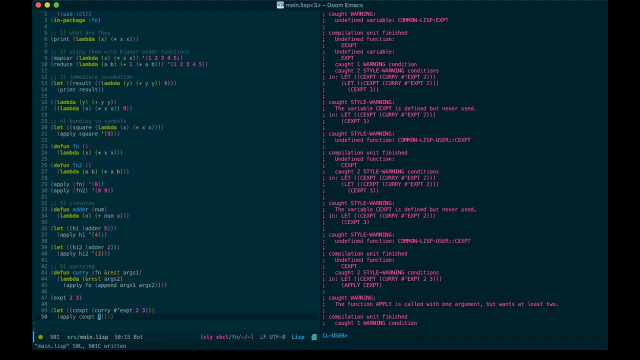 We've actually cast the second parameter into this and I believe, if my logic is correct, it still needs to take an empty argument. that's fine. So we've got this function here. it takes the two and three and using the curry function. 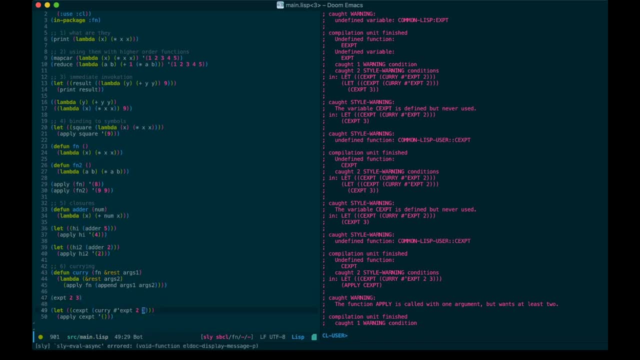 we pass two and three as rest parameters and that forms over and creates a closure here that we now have, and when we apply the result of this closure, we pass in an extra set of arguments. We can then use the apply function again on the original function passed in, which was this: 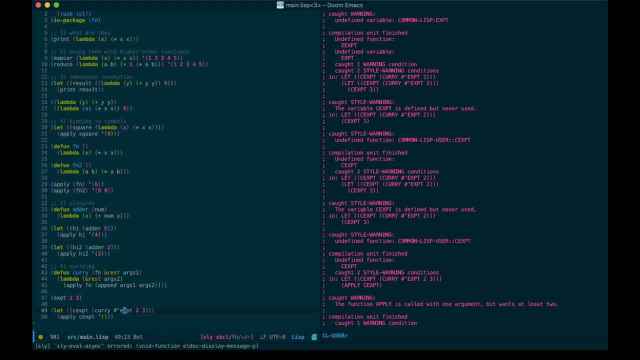 export function and then we use append to join the original argument list with the new argument list and we can get the result. And it's through using this function and returning a function and using apply we can simplify functions down And it might seem a little abstract as to why you might do that, so I'll give you a. 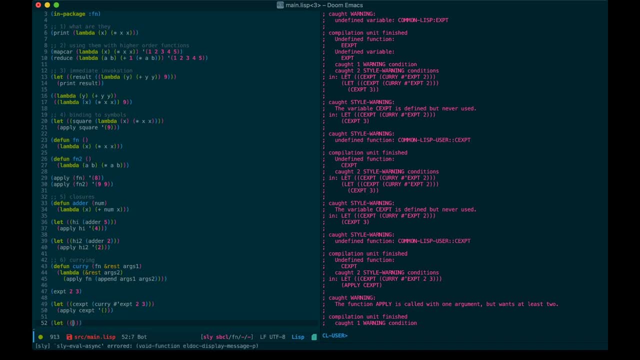 little bit of an example here. Now, let's say that I want to do something in a map car, but my function, that I want to use in that map car, takes more than one argument. We know that the function that map car takes takes one parameter only. 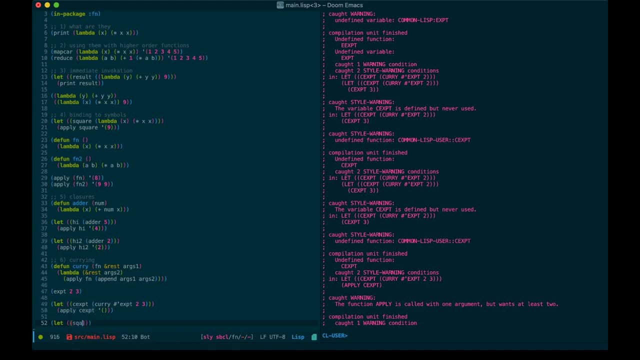 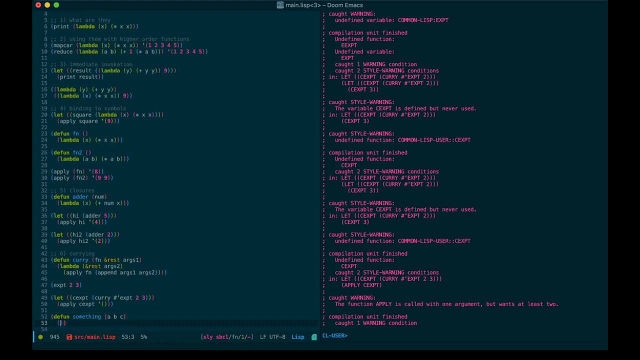 So let's say we've got this square function. Okay, not a square function, some random function defund something. it takes an, a, a, b and a, c and it returns the sum of a, b and c. So it's just going to take three numbers. but 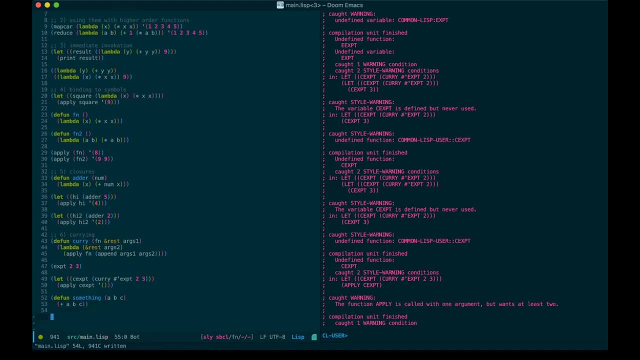 map car can only give us one. So what we can do is we can say let s be the curry, and we're just going to have it add one and two. so we're going to say curry something, one and two. i'm going to make sure that's compiled in that. 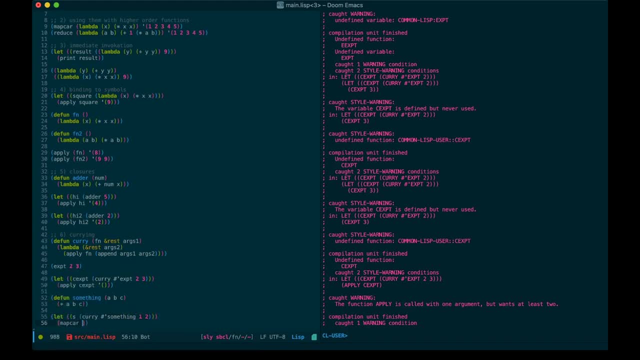 let's say map car s one, two, three, four, five. So we can see here that we've got four, five, six, seven and eight, because 1 and 2 is added to 1, so that gives us 4, and so on, And that's why we get different numbers. 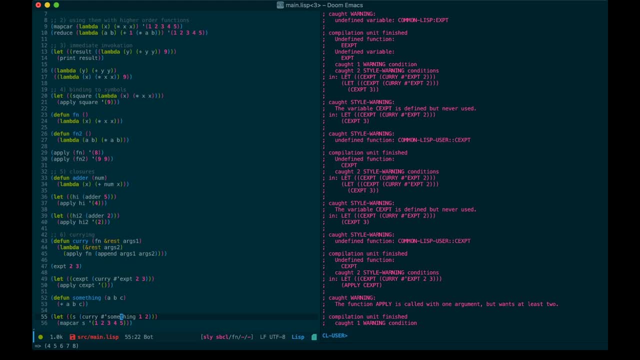 but here we can use currying to actually apply parameters to a function and turn it into a function of a different argument length that we can then chain into using somewhere else. So it's functions and objects and functions being applied a little bit and getting a little bit more. 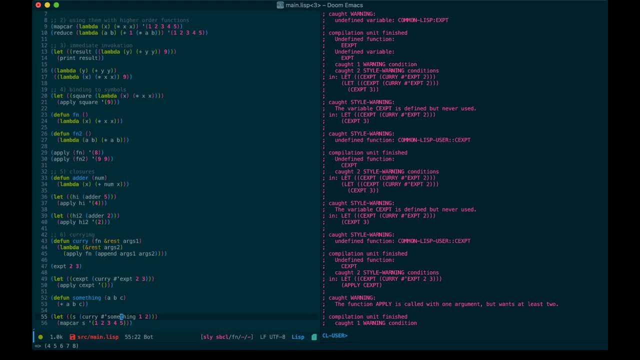 information and a little bit more information until you get a result. And of course you could put like 0 and 0 in here and we'd still get the same thing based on what we know the function is supposed to do. but for whatever hypothetical reason, let's say we just wanted to use this- 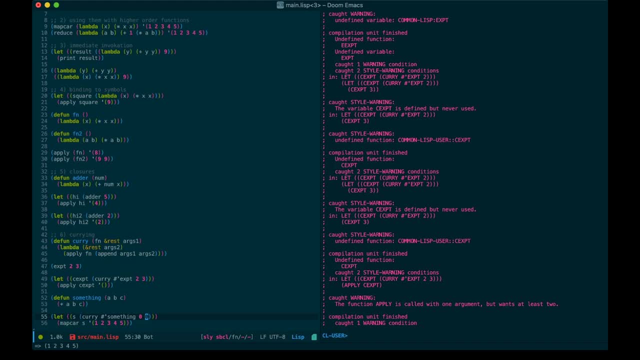 we just pass in some values, partially apply it, understanding the behaviour of the function, and then it just plugs in as ever it would, And it is lambda. that facilitates us using this and that's pretty cool. So I appreciate that was a wee bit of a whirlwind. 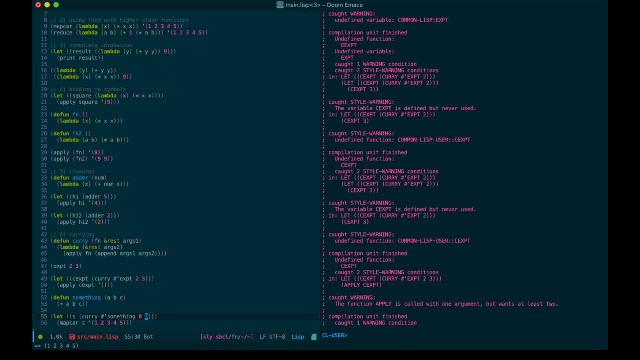 tour through what lambdas are, how you can use them and you know a little bit about what they look like, but there's not a lot more to them than that, And you can curry a regular function, which we did, but you could also curry a lambda, of course. Yeah, that is it. Thank you very much.